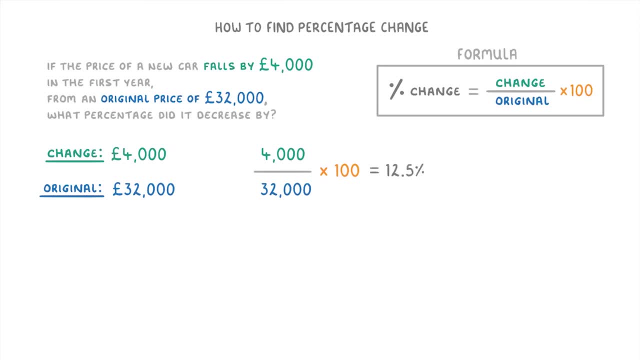 of 12.5% And remember that the price fell, so really it's a 12.5% decrease or we could say that it's a minus 12.5% change. Alternatively, we could have put our change as minus £4,000 to start with. 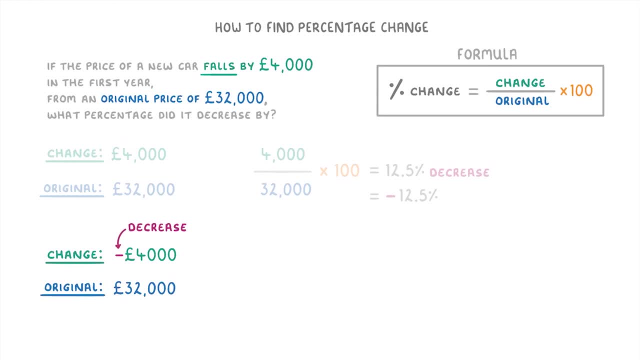 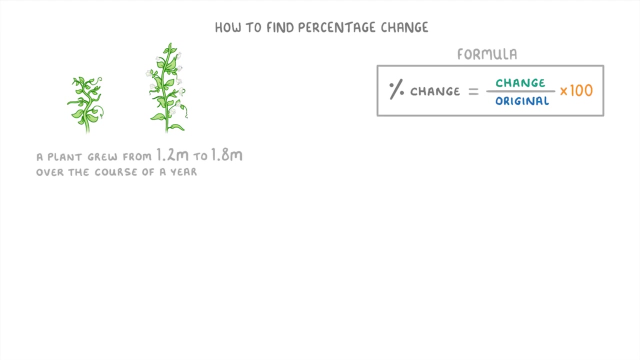 to show that it's a decrease of £4,000.. And if we'd put that in our calculation, then we would have got minus 12.5% straight away. Let's try another one. If I told you that a plant grew from 1.2 metres to 1.8 metres over the course, 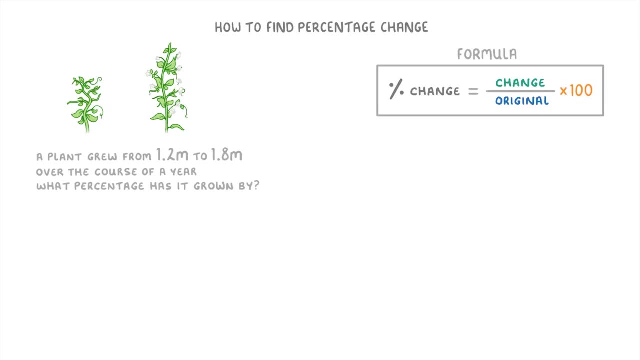 of a year. what percentage has it grown by? Well, if I told you that a plant grew from 1.2 metres to 1.8 metres over the course of a year, what percentage has it grown by? Well, this time we're. 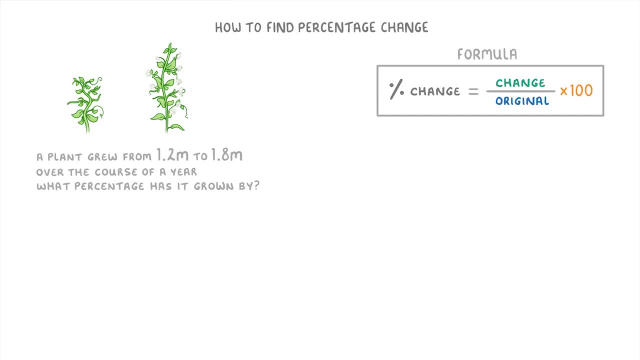 not actually told what the change is. We're just told that the height changes from 1.2 to 1.8.. So we're going to have to calculate the change for ourselves by doing 1.8 minus 1.2 to get a change. 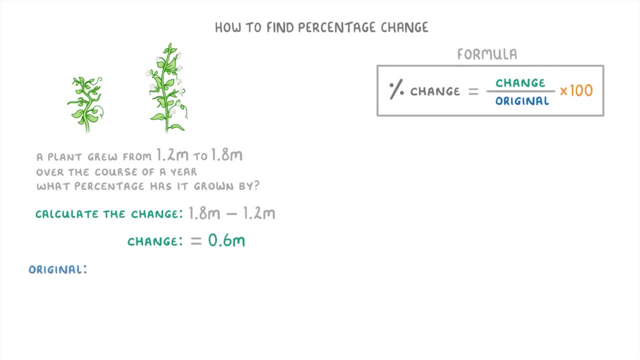 of 0.6 metres. Then the original part refers to the height that the plant grew from or started at, So in this case, the 1.2 metres. So, overall, we do our change of 0.6, divided by our original of 1.2, and then times it by 100,. 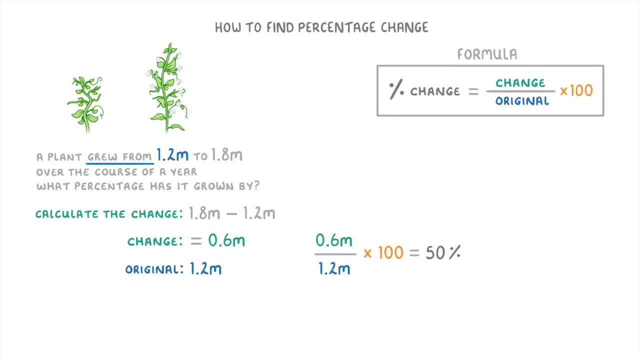 which is 50. So the plant grew by 50% over the course of the year. Have a go at this last one. So this time we're told that a cat starts off weighing 0.7 kilos. Then, 8 weeks later, 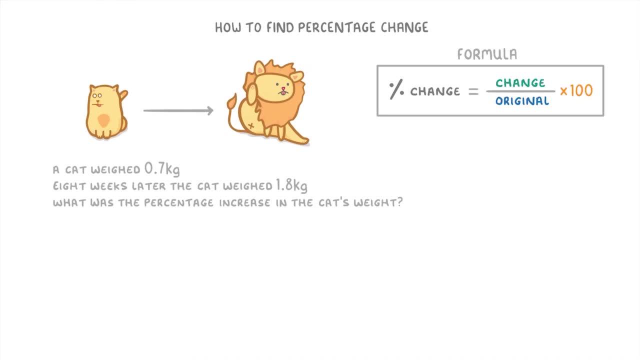 it weighs 1.8 kilos And we need to calculate the percentage increase in the cat's weight. This time, the change will be the difference between the two weights, which we find by doing 1.8 minus 0.7.. So 1.1 kilos. 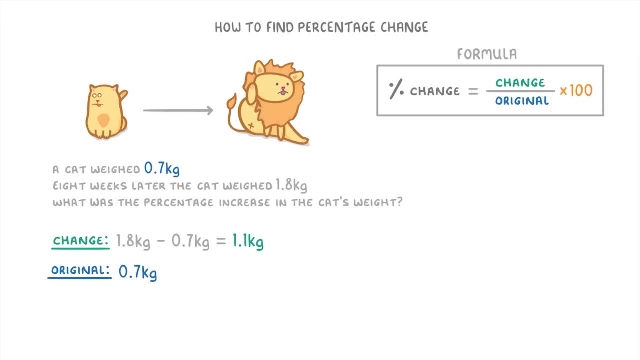 And the original will be the 0.7 kilos that the cat started at. So for our working we do 1.1 divided by 0.7 times 100, which, when rounded to a whole number, is 157%.